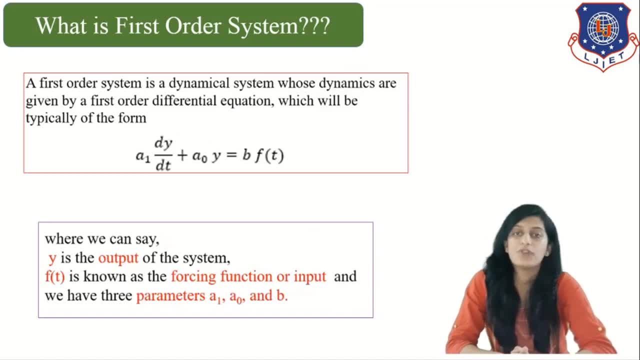 So, basically, what do we mean by a first order system? A first order system is a system or a dynamical system whose dynamics are given by first order differential equation In simplest form. if I want to explain a first order system, then it can be defined as a system. 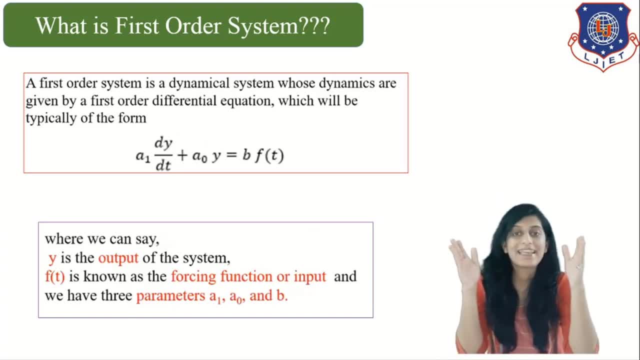 whose input and output can be correlated with each other or can be represented in the form of a first order differential equation, then such equations or such systems are termed as first order system. So when we are talking about a first order system, representation of a first order system is given. 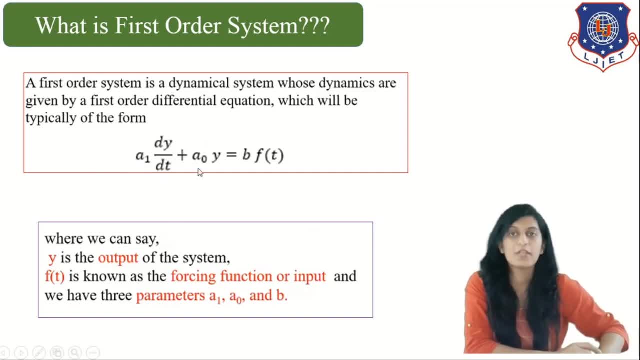 by a, 1 dy, by dt plus a, 0 y equals to b, f of t. So what do we mean by y here and what do we mean by f of t here? right? So y which is denoted here is our output, the output which is coming. 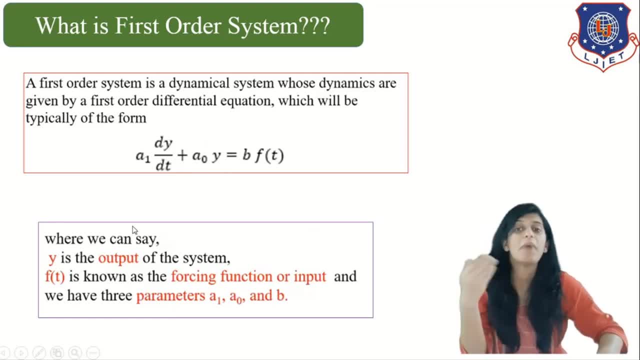 out of the system or the output which is given by the system is denoted by y. f of t is basically a forcing function, or it is also known as input function, the input which we are giving into a system. A, 1, A, 0 and B are parameters of the system right. So whenever we can relate input, 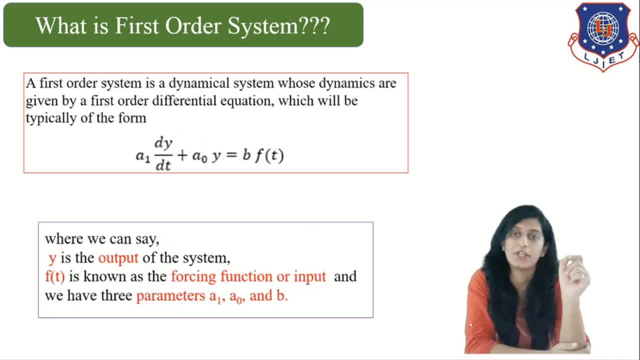 and output using a 1 dy by dt plus a 0 y equals to b f of t, then it is denoted by y. So when we are using first order differential equation, then such systems are termed as first order system. There are many examples of first order system, such as mercurian glass. 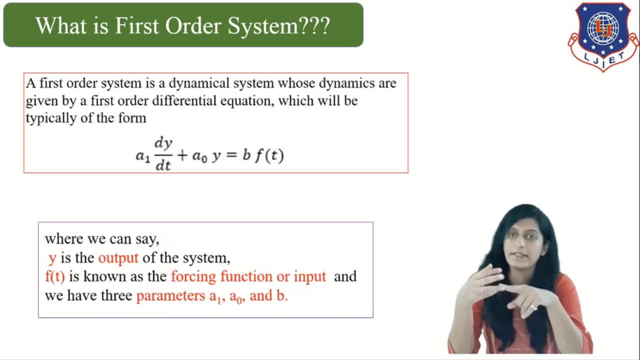 thermometer, liquid level system, heating system, interacting tank and so on. right, So one by one, we will derive and see how they are. their input and output are going to be correlated with each other, and what are the various parameter which actually affects? 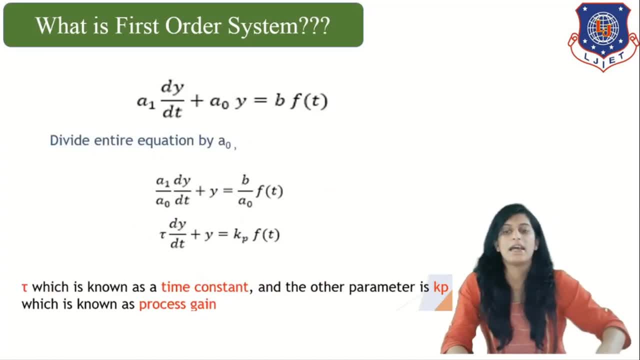 those systems And, as you can see here, so A 1 dy by dt plus A 0 y equals to b t. this is our equation. So if I divide the entire equation, u by A 0, so it will be A 1 by A 0 dy by dt plus y, because A 0 by A 0 is 1 equal to A 0 by. 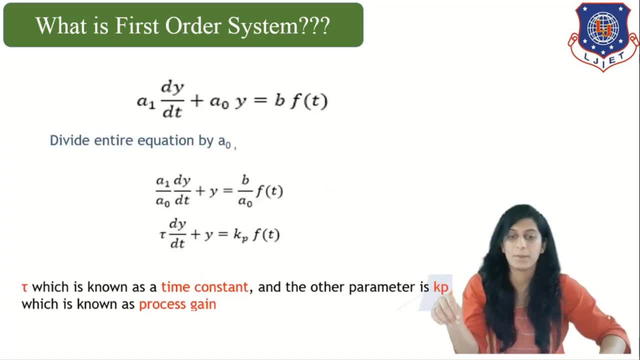 A, 0 is 1.. equals to f of t. Now again, a1 by a0 can be written as tau, So b by a0 can be written as kp, So tau. here is our time constant and kp is actually the process gain. This is how you. 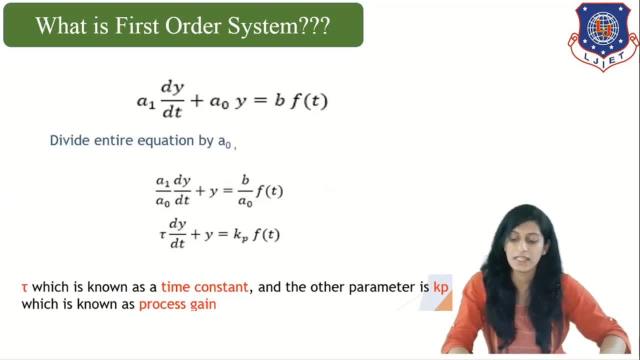 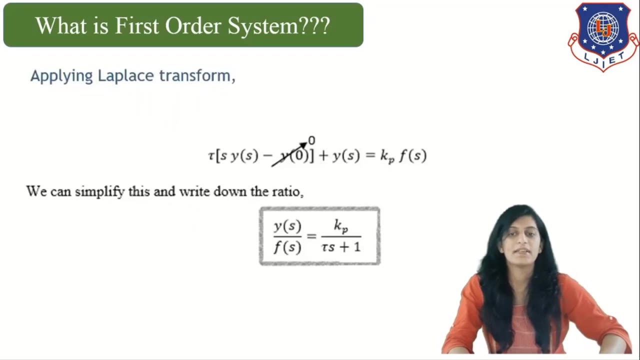 represent first order system of any first order equation of any system right. This is representation of first order system. Now, if you apply Laplace, So it can be tau: s y of s minus y0 plus y of s equals to kp f of s right. So if you take y of s common and shift the term, 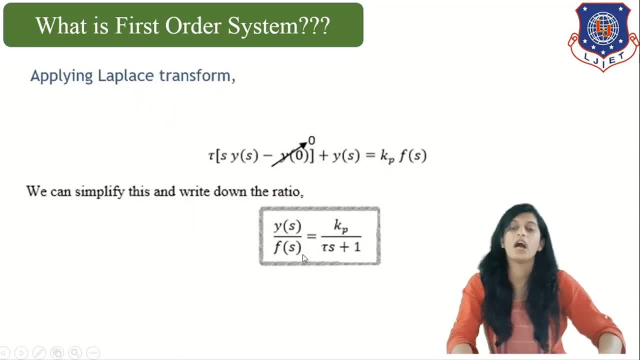 you will be getting y of s, which is our output, upon f of s, which is forcing function. So y of s is a function of, or our input equals to kp upon tau s plus 1.. So this is basically the simplest form of representing first order system and it is known as transfer function. 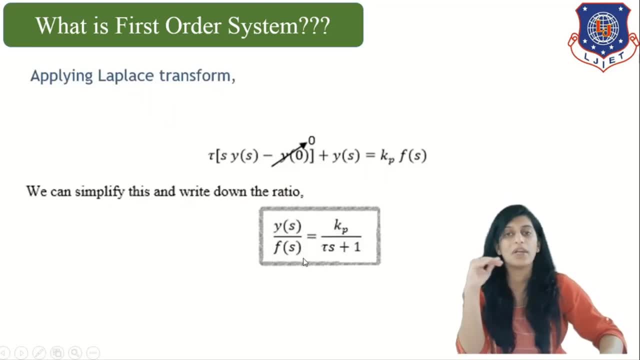 Transfer function means a ratio of output upon input of any given system. So this is our transfer function for first order system, Where ys is the sphere of first order system: 1. s is output, f of s is input, k, p is gain, tau is time constant, s plus 1.. 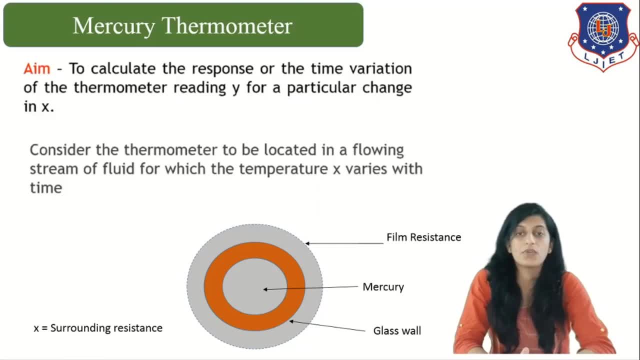 Now let us start our today's first derivation, which is mercury thermometer. As I already informed you that mercury in glass thermometer is example of first order system, That means its application or the way it works can be represented in the form of first order differential. 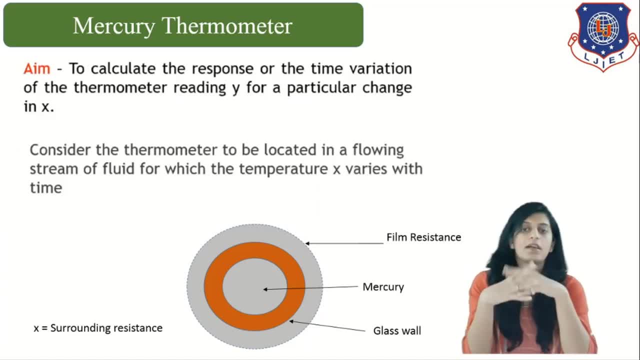 equation. So let us just start. We are going to derive a relationship between output and input for mercury in glass thermometer. Now, as you can see here, what is our aim? Our aim is to calculate the response or time variation of thermometer. 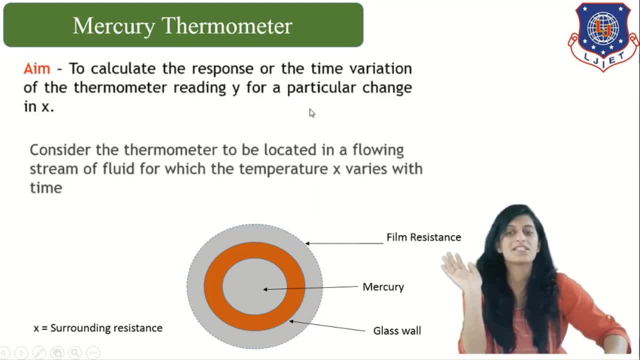 Reading y for a particular change in x right. So let us just consider that a thermometer is located in a flowing stream right And the temperature of that flowing stream is x right. So, as you can see, this is our bulb of thermometer. This is the inside portion. is mercury. 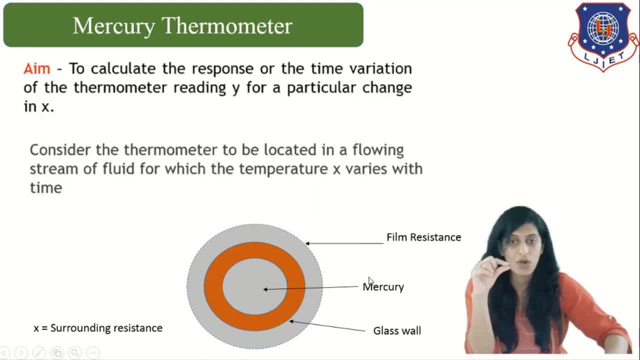 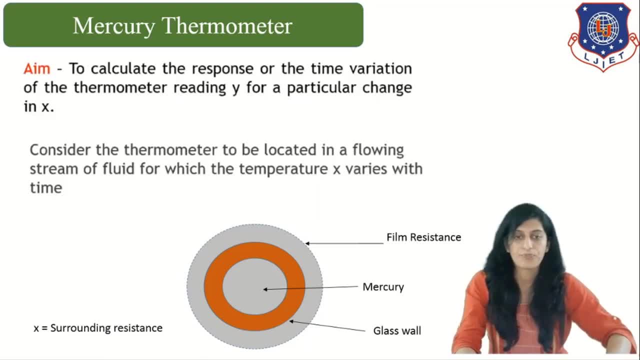 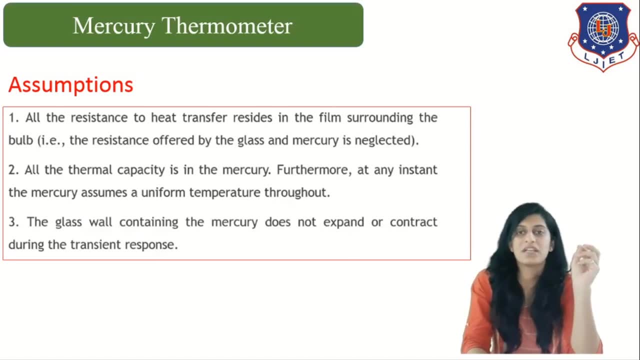 is being immersed. Now, as we all know that for any derivation we must do some basic assumptions right. So in mercury, in glass thermometer thermometer, we are having three different assumptions. First one: all the resistance to heat transfer resides in the film surrounding the bulb. That means the resistance which 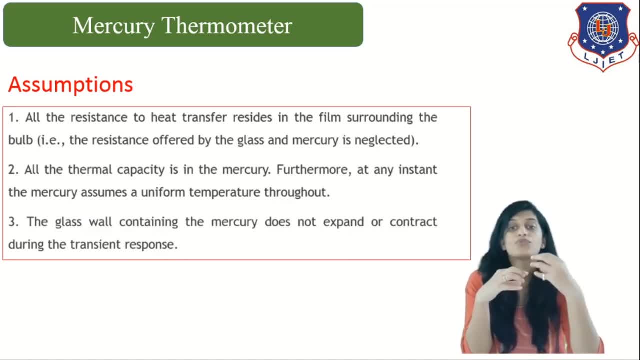 is offered by the glass of thermometer and mercury is neglected. So we are assuming that there is no resistance to heat transfer from bath to the mercury. Second assumption is: all the thermal capacity is in the mercury. Furthermore, at any instant, it is assumed, 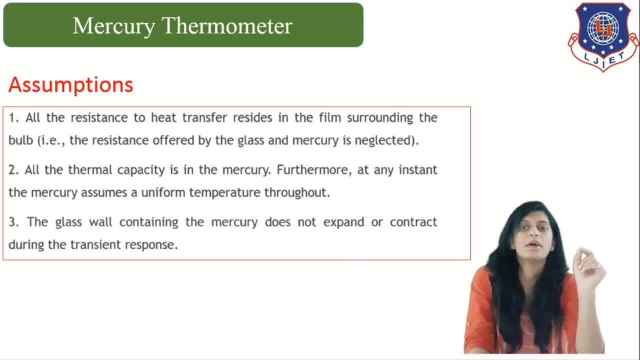 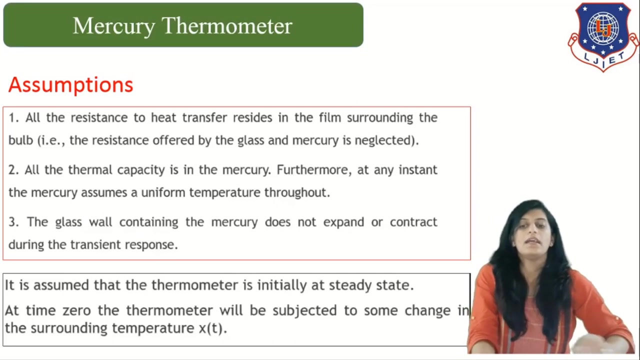 that mercury will have uniform temperature throughout. right, We are assuming that mercury is having a uniform temperature throughout. The third assumption is the glass wall of thermometer will neither contract nor expand. So these are the three basic assumptions of this particular derivation. Now it is. 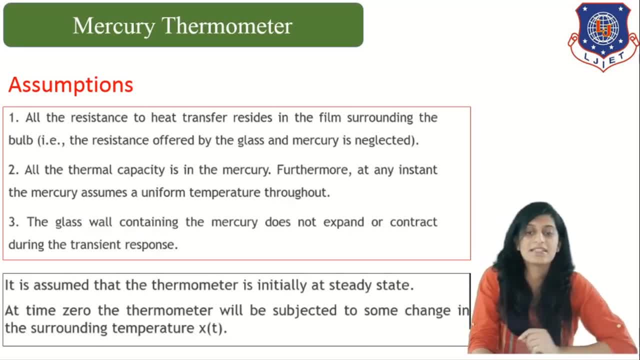 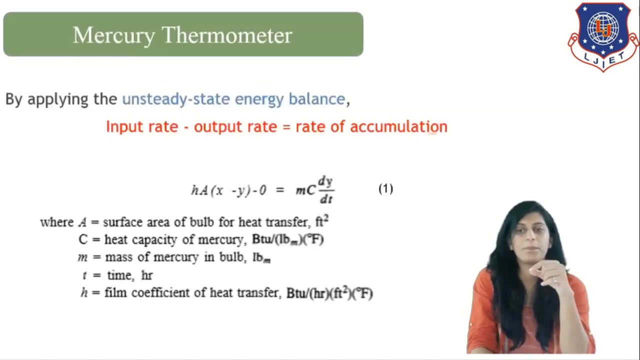 assumed that thermometer is initially at steady state and when time is 0, initially we are keeping thermometer at steady state, That is, at room temperature- Then at some given time t equals to 0, we will immerse that thermometer in a bath of fluid which is having temperature x of t. So now what we can do. 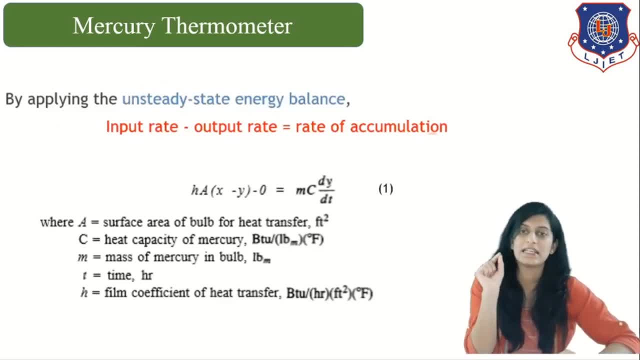 is we will be applying unsteady state energy balance. Why we are applying energy balance? Because this is a case of energy transfer, right Heat transfer. So we are applying energy balance. So, as you can see here, input rate minus output rate equals to rate of accumulation. 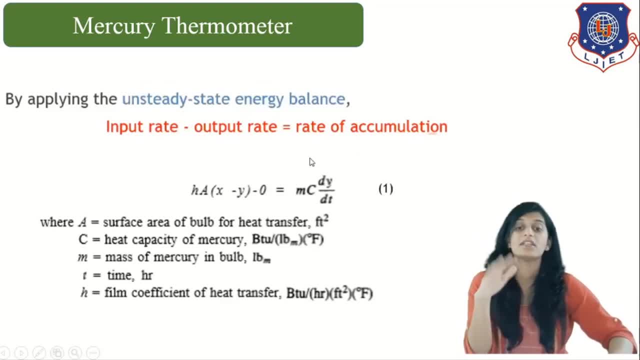 Now in mercury, in glass thermometer, there is no output in physical form, right? So output term will be 0.. So what is input Input? is h a delta t, right? So h a delta t, So h a delta t. 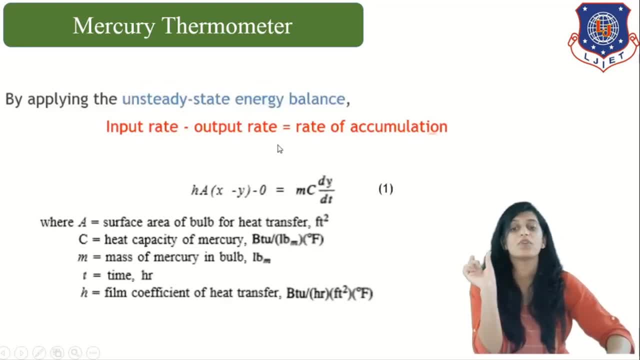 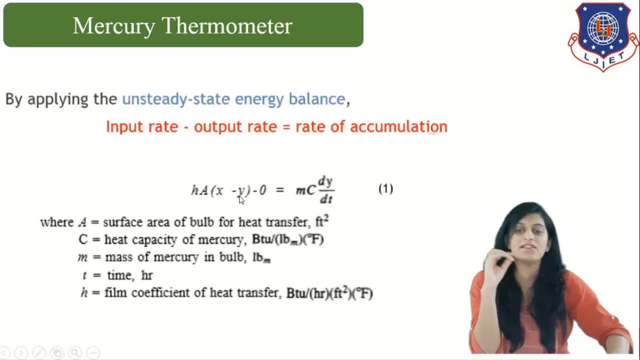 t. So h a delta t y. Thus, if h a is equal to 0,, then input of holiday is equal to 0.. And what about temperature of bath? It is minus because of temperature of temperature of bath. The difference 그게 the difference in temperature. how much heat will be going? 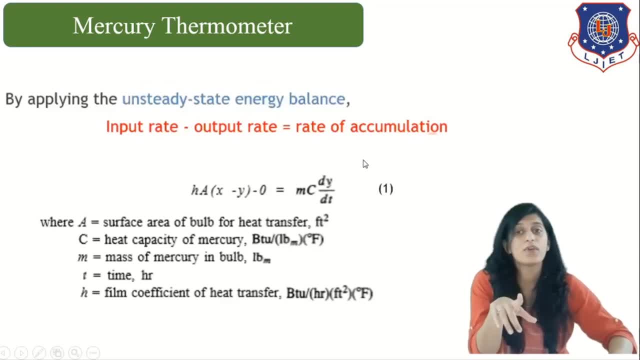 inside temperature of bath, minus temperature shown by steady state thermometer, So x minus y. So input is given as h a, x minus y and rate of accumulation where the heat is going to accumulate inside the mercury. So m cp delta t will be 0, right, So we have a temperature. 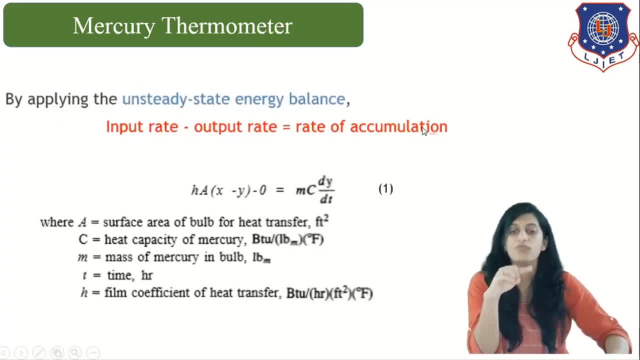 of 4 degrees centigrade. So if we investigate where education of, OF course, documentary É rate of accumulation, So M, C, p, delta, T can be given as change in thermometer reading which is dy by dt. So as you can see, A is our surface area of bulb for heat transfer, C is our heat. 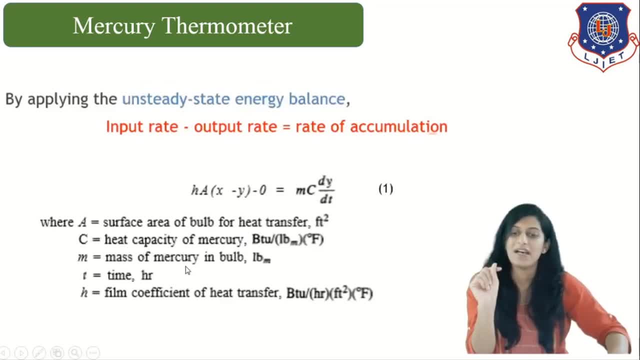 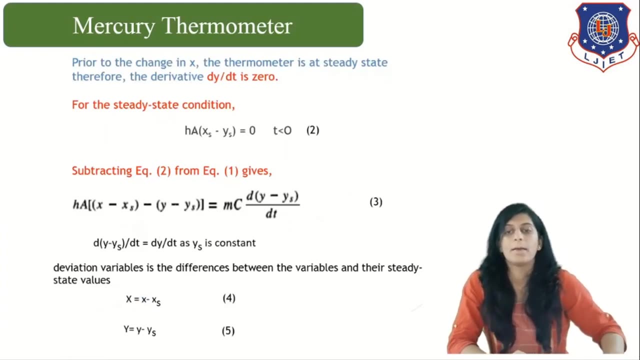 capacity of mercury. M is mass of mercury in bulb and T is time. H is film coefficient of heat transfer. Now let us just say we are going to apply steady state condition to our heat energy equation, The equation which we have obtained, that is, 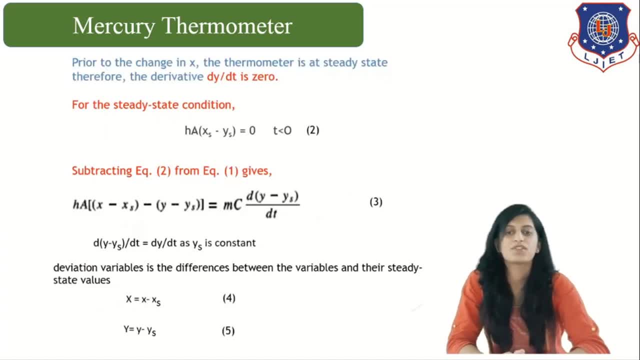 H A, x minus y equals to M, C, dy by dt. Just apply steady state to that equation So it will reduce to H A, x of s minus y of s. This small s in suffix shows steady state condition right Equals to 0. 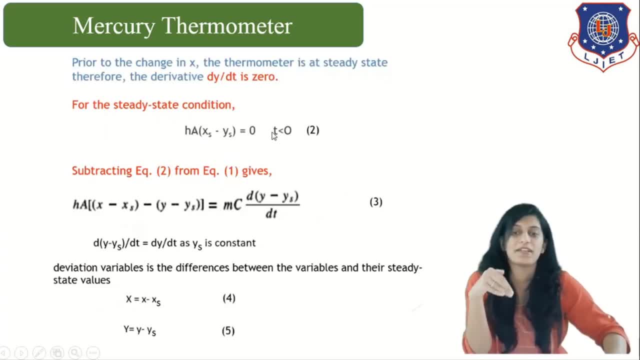 Why 0?? Because anything which is changing with respect to time, that is, constant value at steady state variables are constant. So dy by dt is 0.. Now we will subtract this steady state equation from this equation. So we will subtract this steady state equation from this equation, So. 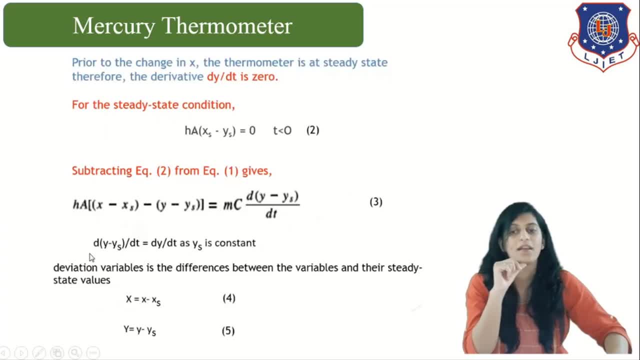 we will subtract this steady state equation from unsteady state equation, that is, equation number 1.. So it will be H A x minus x of s, minus y, minus y of s, which is equals to M C dy minus y of s by dt. We can substitute y of s because dy s by dt is ultimately 0, right, Doing this and introducing 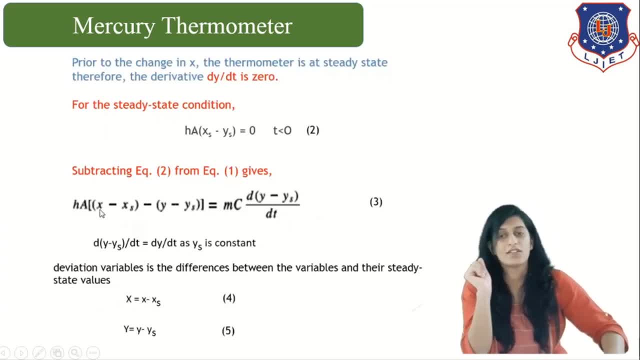 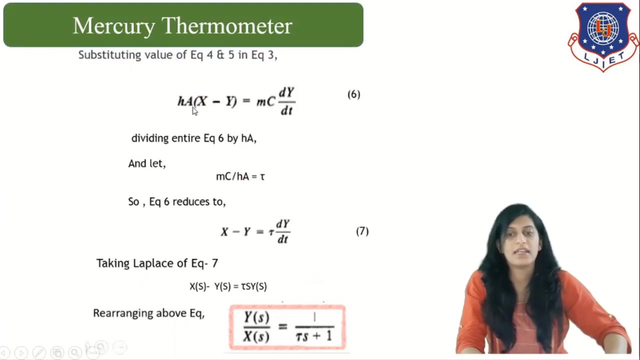